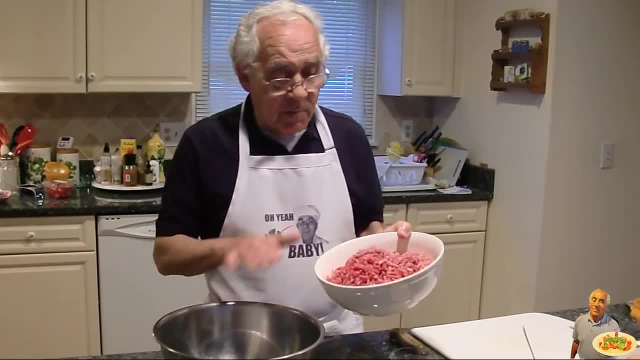 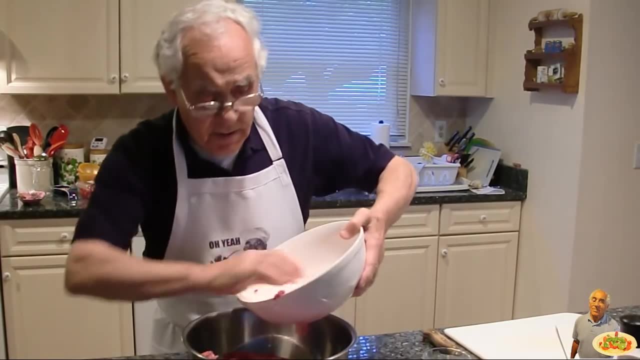 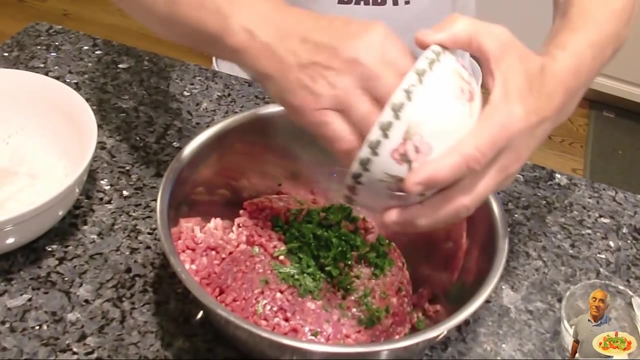 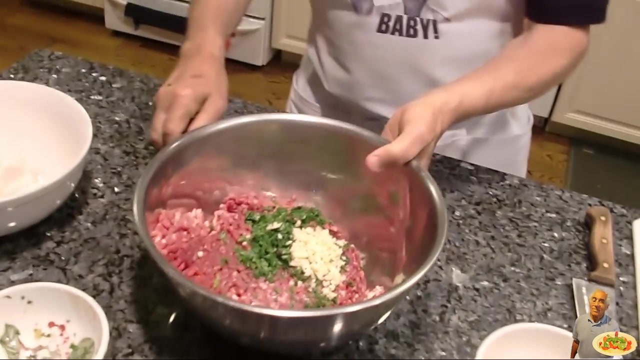 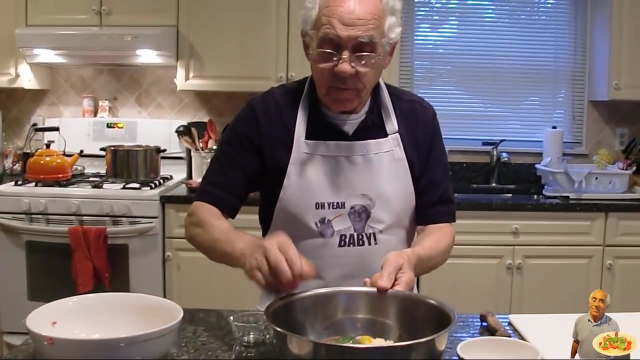 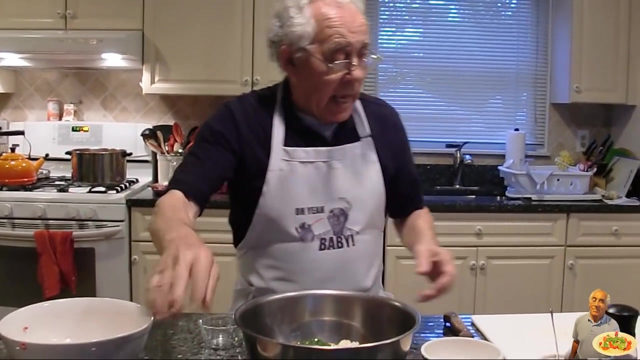 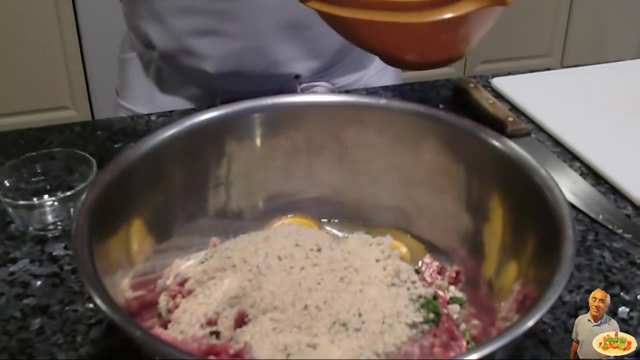 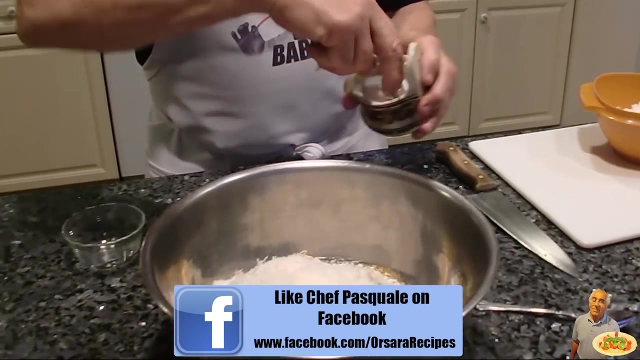 myself with a machine. Now we start putting the meat over here because this dish is too small. I put everything on this one. Now. I use parsley garlic. Now we put three eggs- One, two, three- And I use breadcrumbs And I use a Parmigiana cheese, Salt And black pepper. 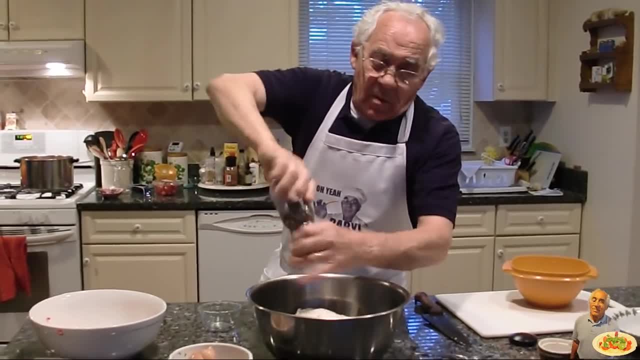 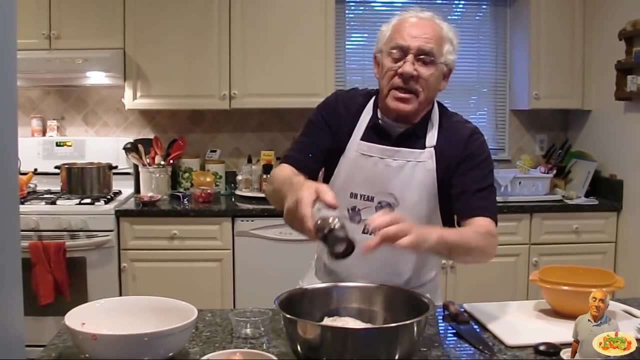 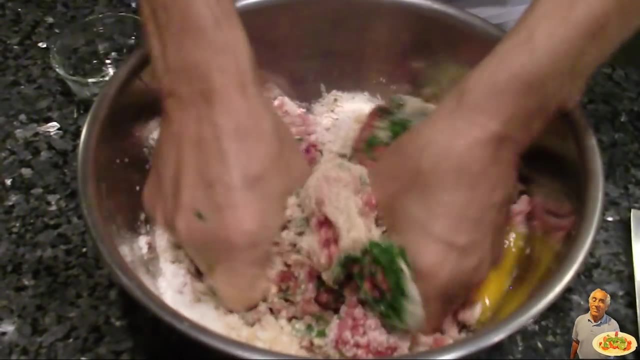 And I use. no, I got my sauce Already made. I want to show the sauce, the sauce I was making After I put the meatball. Okay, now we start the mix. I'm washing my hands already And we mix, You gotta. 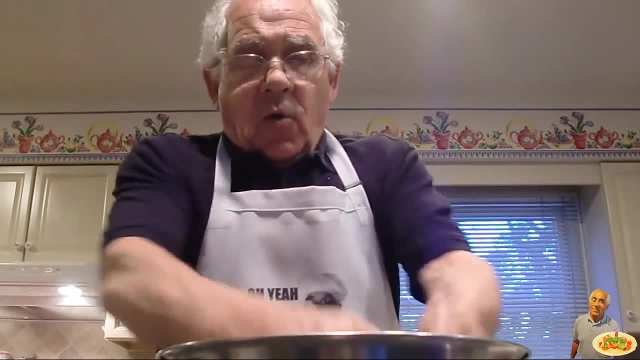 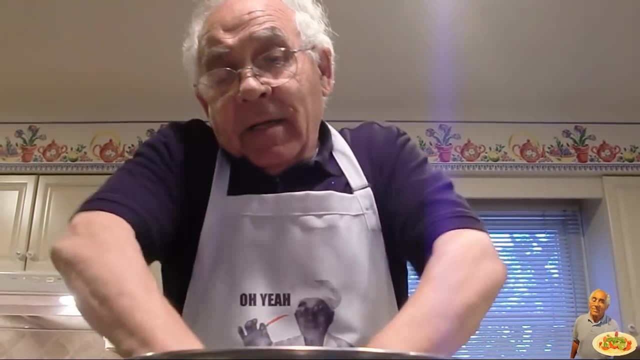 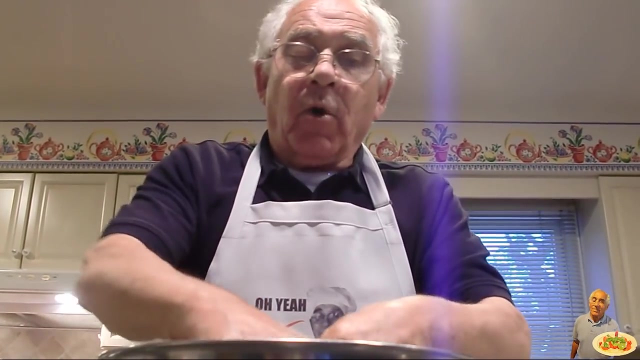 mix really good. When it's mixed good, you gotta make sure the taste. you know a lot, a lot in a lot like to taste the meat, the raw meat, but I always eat it all the time I work at a. 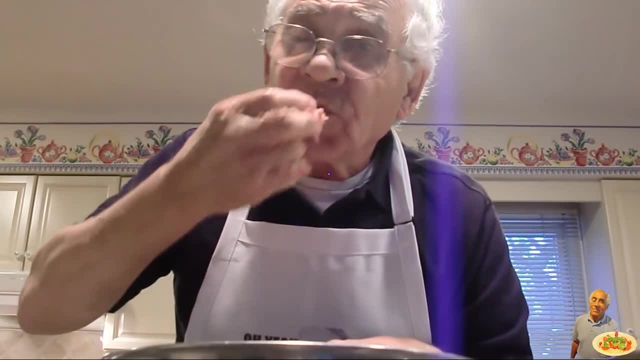 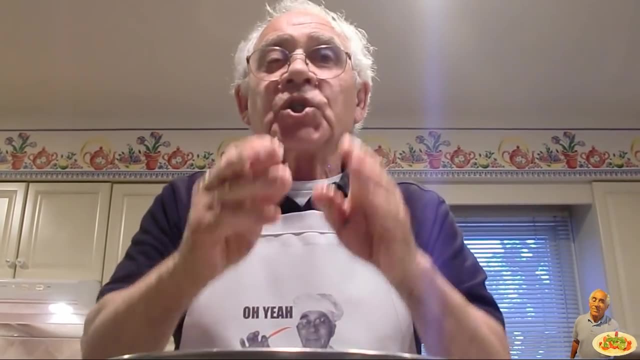 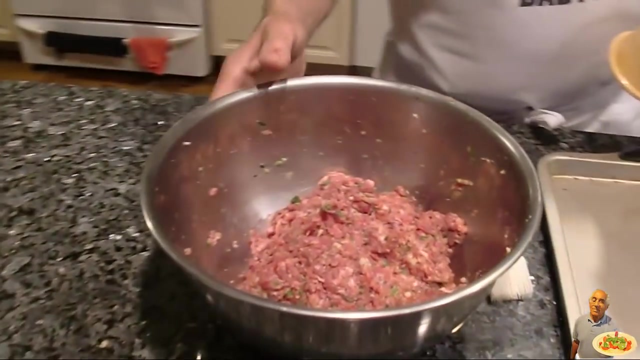 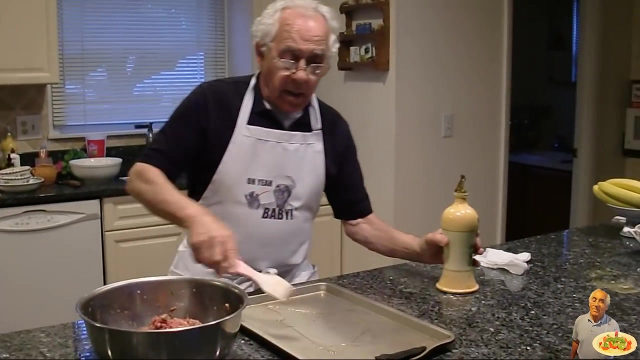 restaurant. I always taste all the time the raw meat. It's perfect. Salt, black pepper, cheese, eggs- it's a really good taste- And the garlic. Okay, now the meat is all mixed together. What I do? I put a little drop of the oil and I brush. 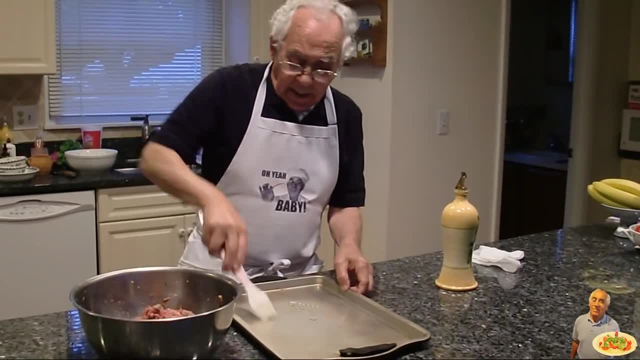 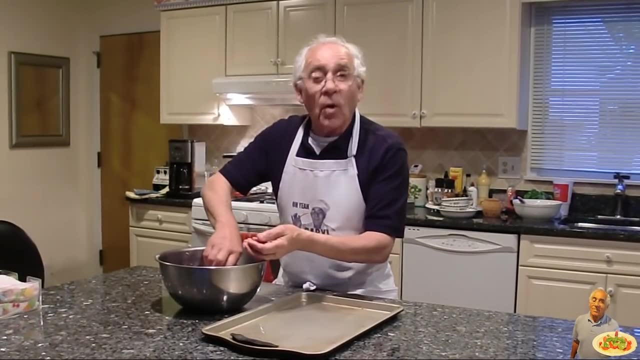 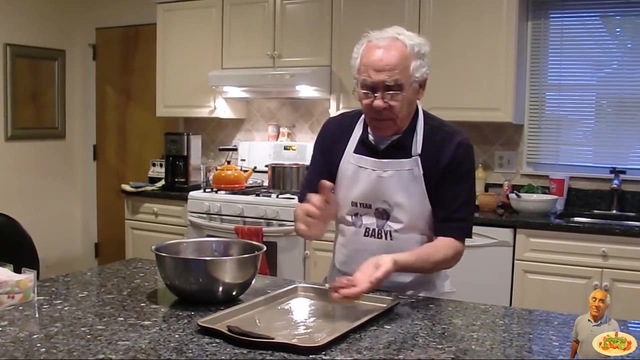 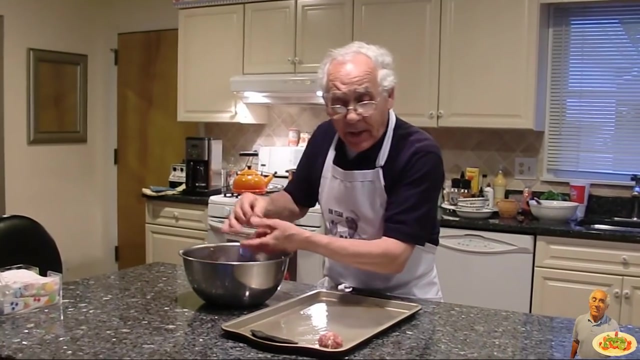 underneath the parts like this: A nice time to roll it. I don't like big, big meatballs. I like the meatball this size, like this You put right over here, and I put the oven on four, four, four hundred degrees, because when the meatballs are ready I put them on the oven about 15 minutes. 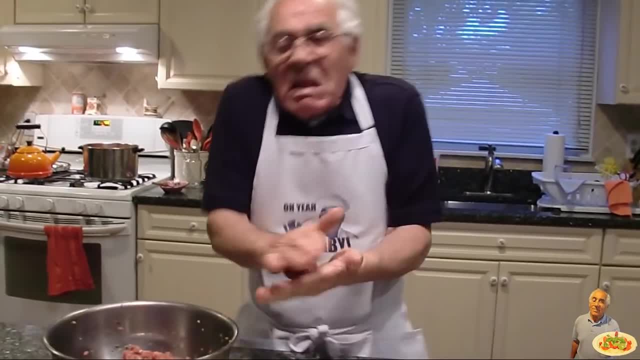 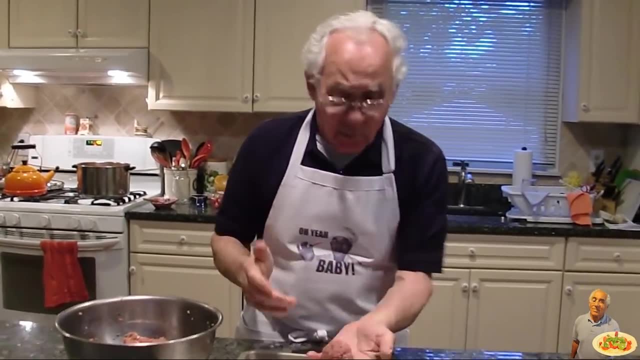 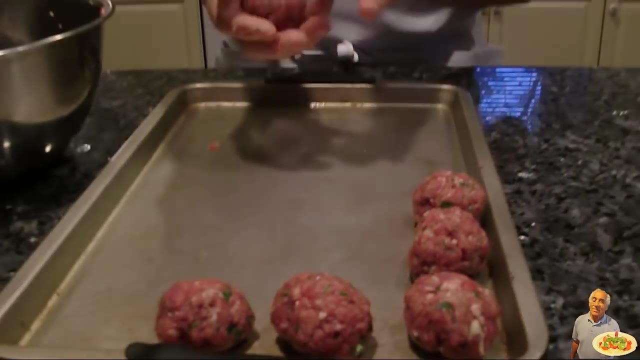 And look when I roll, it's not you gotta do like this, you gotta roll like a boss like this. you see, If you don't squeeze it, it comes really like a baseball. look at that Now the restaurant. what it do, it make a really big meatball. This, you gotta make the meatball. 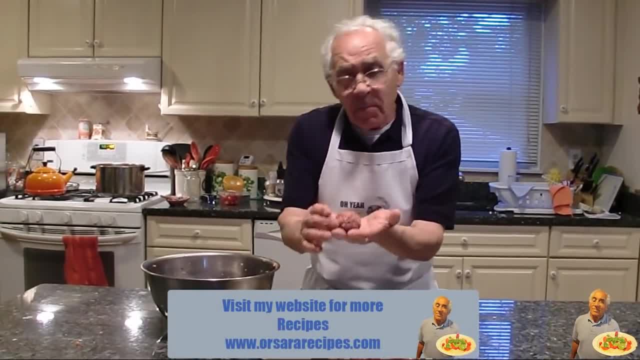 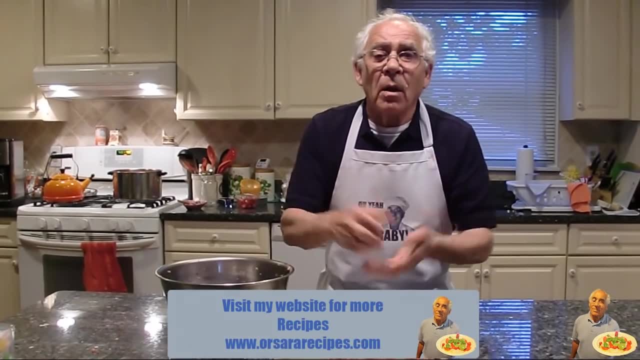 nice size. you go eat a dish of spaghetti. you can put maybe three on the top. You go to the restaurant and every time you give it to you one, it look like a soccer ball. This you gotta be like a golf ball. 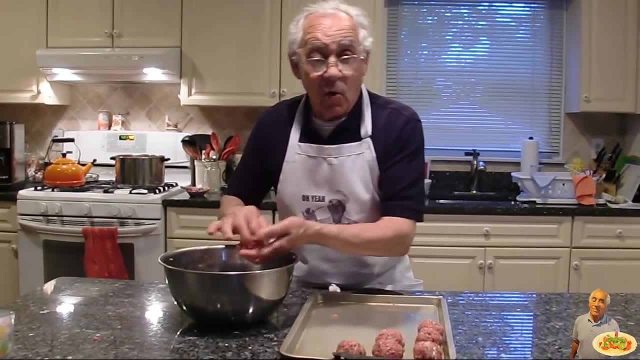 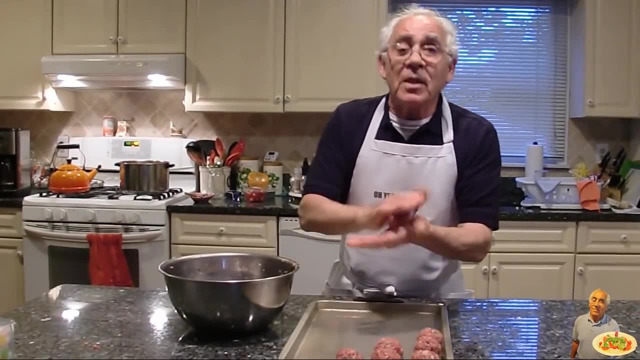 like this small, a good sauce. Wait when I show you the sauce I make over there. I got nice big parts over there ready. When you eat this, all the juice of the tamari go inside. it's so soft you can make. 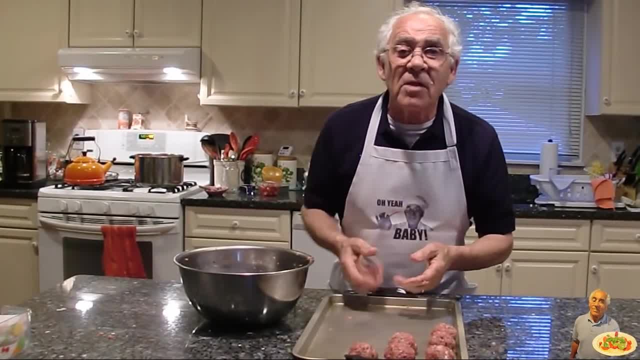 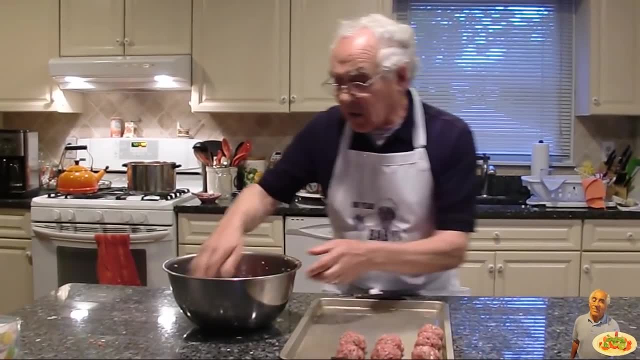 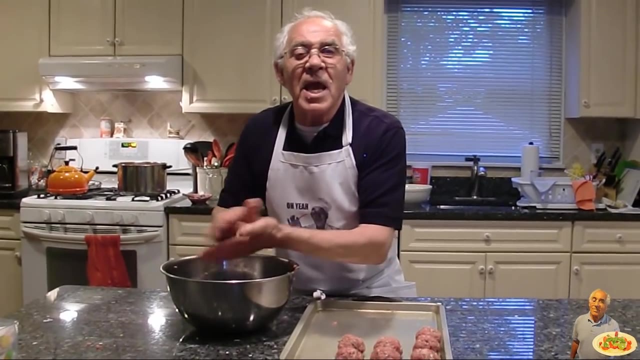 something: Sanmarino: meatball, the sauce on the bread, three meatballs like this, the food Sanmarino, three or four meatballs and with the sauce it's so good It can look on the TV- your football game, basketball game. you don't gotta order from. 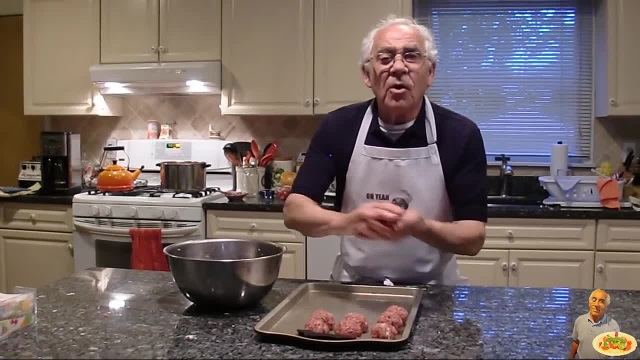 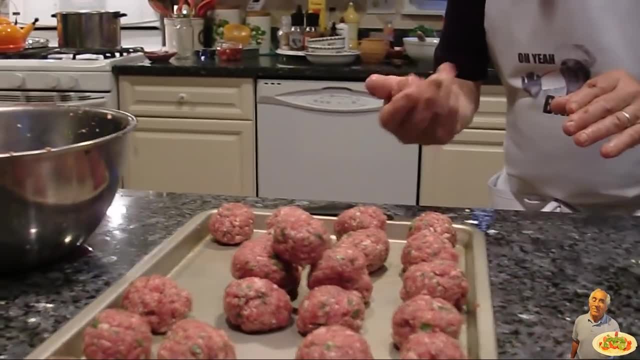 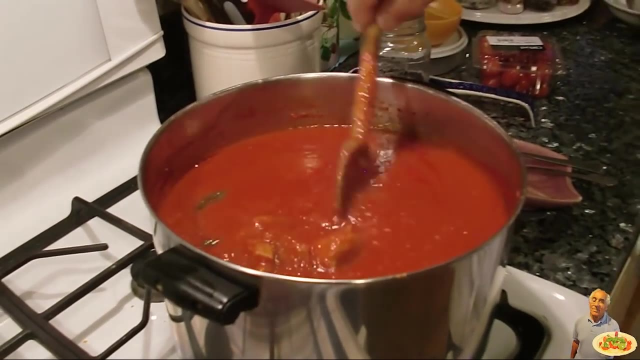 nobody, you make it by yourself. look And you roll and you boom. It's so easy. Now, with this meatball, we can play Bacce Boom. I got two points Now. this is the sauce I was making today, and I cook the pork. 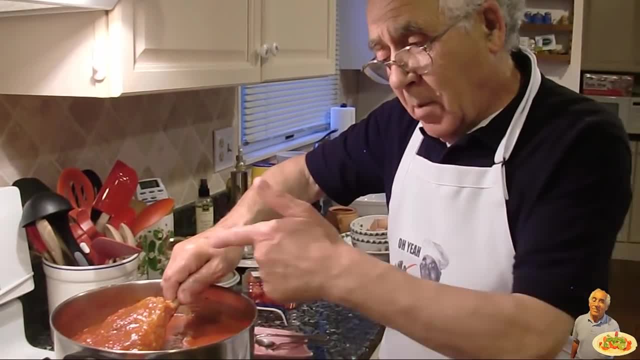 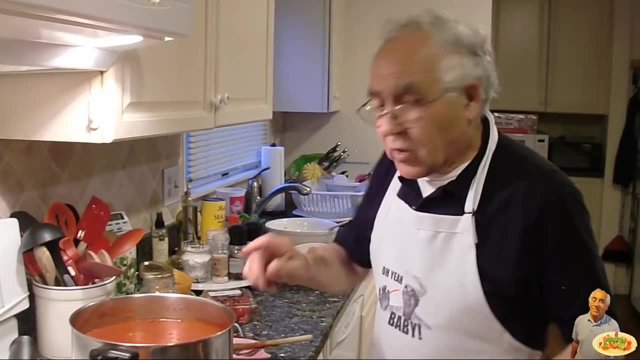 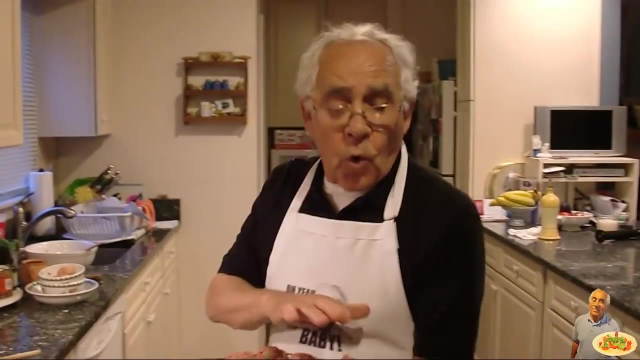 bones inside with the meat and the meat I take it out for this. I was making the meatball. Now it's time that put the meatball in the oven. You got to stay for 15 minutes. You don't got to cook all the way After. I got to cook in the sauce for 20 minutes. 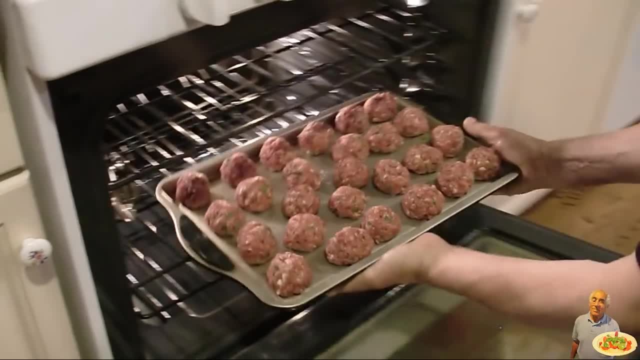 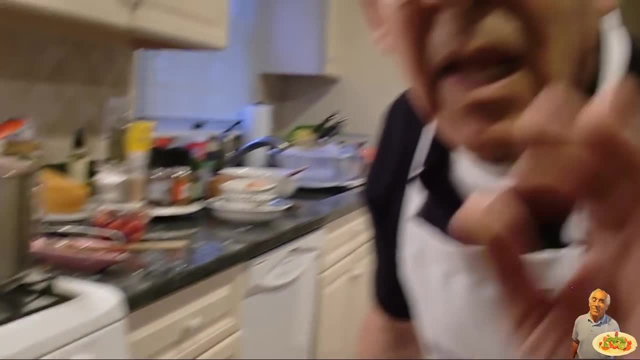 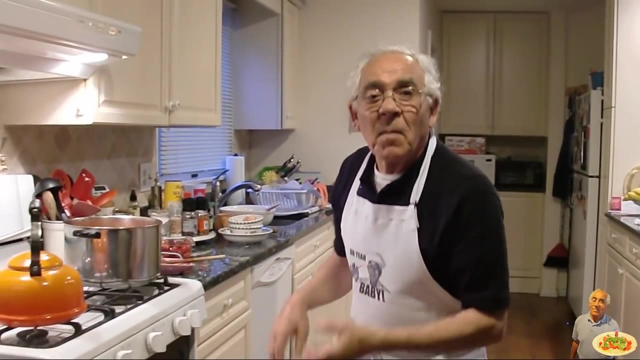 Now we put it in the oven After when this is done. you got to smell this. It's a shame nobody can smell on the camera, but I can smell over here my cheese, my garlic, my parsley- Everything smells so good.